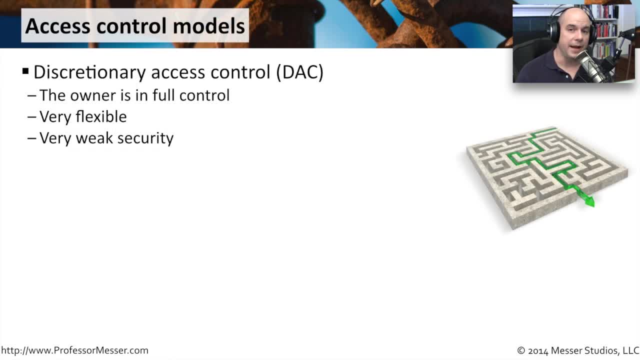 or a mandatory access control. With discretionary access control, the person who owns the resource is in complete control of who might have access to that resource. It is very, very flexible, but from a security perspective it's very weak. You have the person who owns that information now making. 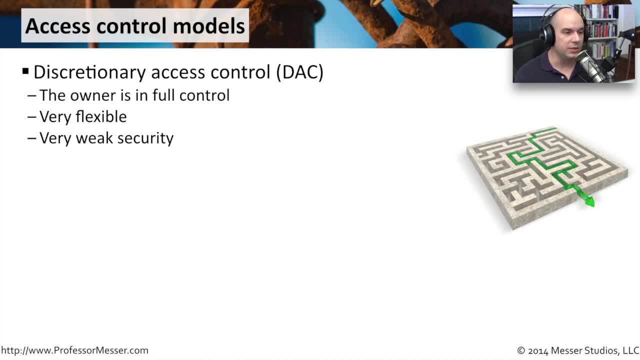 security, decisions on who gets to access it And one small slip from the owner. the owner could give full control to everybody and not really mean to do that. A step up from that is role-based access control. This is where we are defining what access. 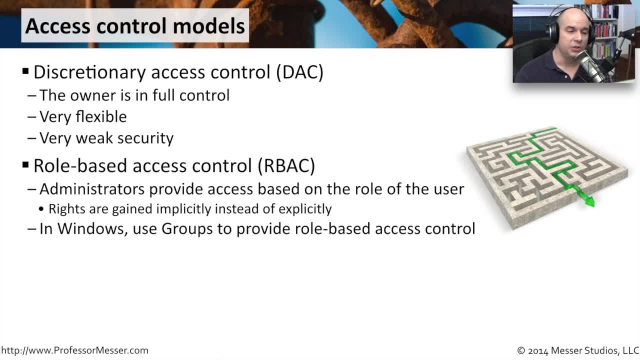 you may have to a resource based on the role of the user. So you may be in a group of people, You may be in a department, You may be part of a team of people And we'll say that if you're on this team. 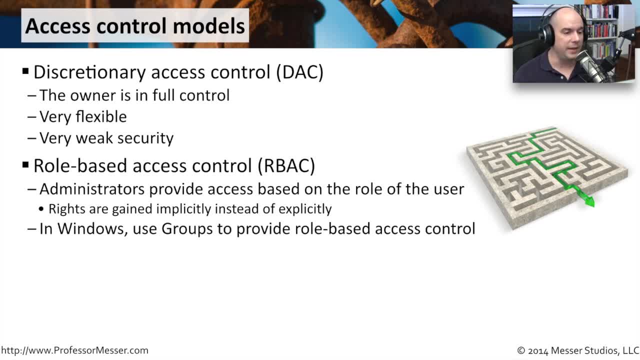 you have the ability to read these particular files. This role-based access control also gives you a little more control over what's going on. It scales a little bit well. In Windows, we use groups to be able to accomplish this, So you would add all of these different users to a group. 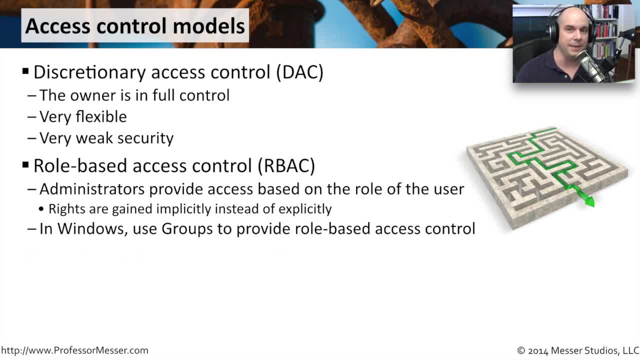 and you would simply assign rights to the entire group at one time. We often see mandatory access control used in government-type environments, where there are security clearance levels And everything that you would need to access would have a label associated with it: Every document, every printer, everything. 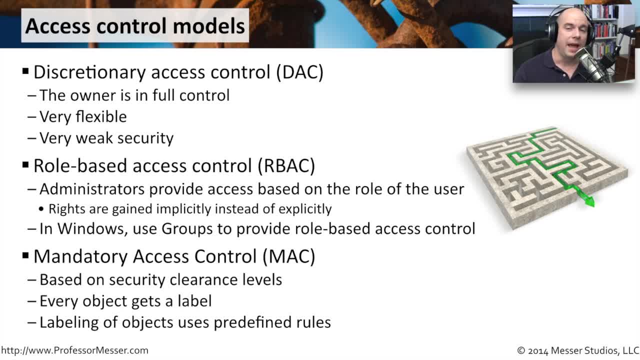 would be labeled with secret or top secret or code blue, And your account would be given a certain level of access. Your access may be able to access top secret, which means you could access anything labeled with top secret or secret, because that's one level underneath. 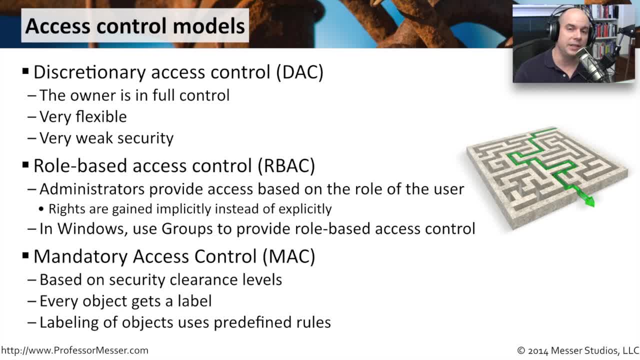 But you would not be able to access anything that was code blue. It's an interesting approach to being able to control what's out there and make sure that only the certain people associated with that level of clearance would have access to those resources. You may hear access control referred. 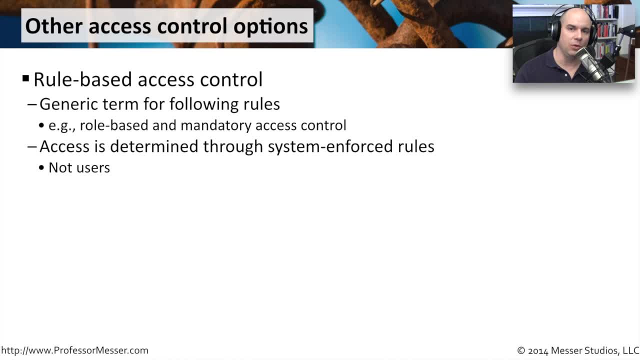 to as rule-based access control. This is more of a high-level way to describe the way that rights and permissions are given. One type or two types of rule-based access control is role-based and mandatory access control, Because those access control methods.